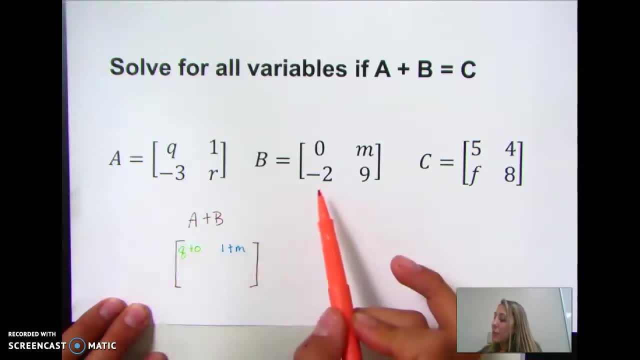 I can combine these like terms. So negative 3 minus 2 is negative 5.. So I go ahead and combine those. So that would be there, And then let's see what color I'm going to use. this one, All right, and then I'm going to do R plus 9.. 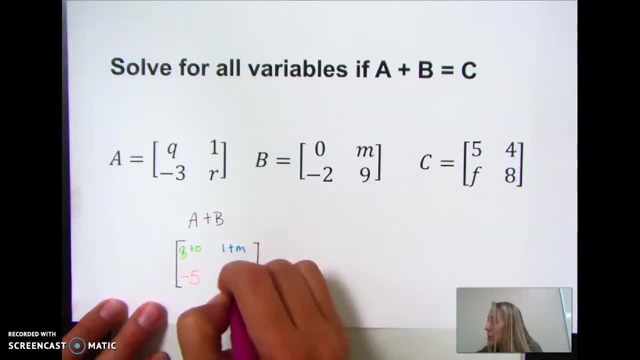 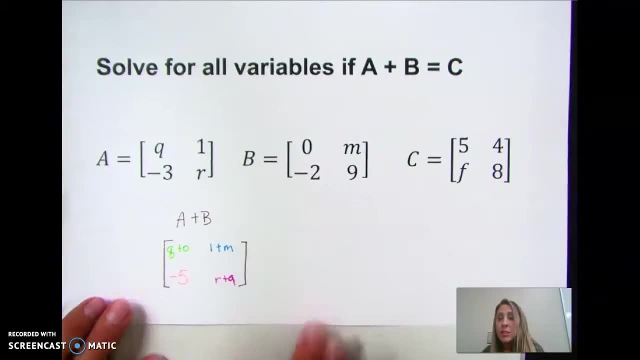 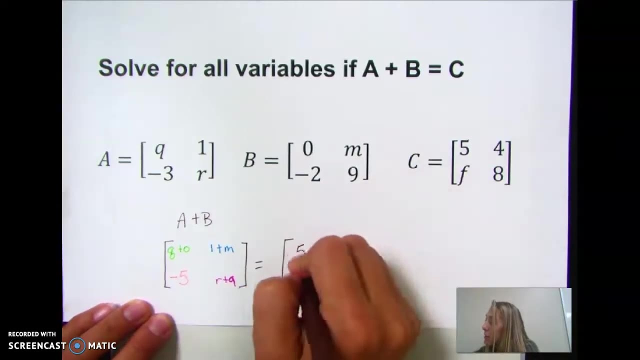 Again, those are not like terms, So I'm just going to write R plus 9.. Okay, All of that is going to equal matrix C, So equals. and then I'm going to write my matrix C, 5,, 4,, F and 8.. 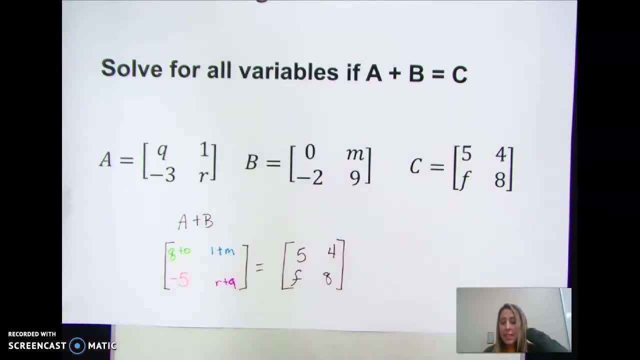 All right. so now to solve, all we have to do is take each thing with a variable and set it equal to whatever this is. So, just like adding and subtracting, I'm going to take the Q plus 0, equals 5, and I'm going to set that up. 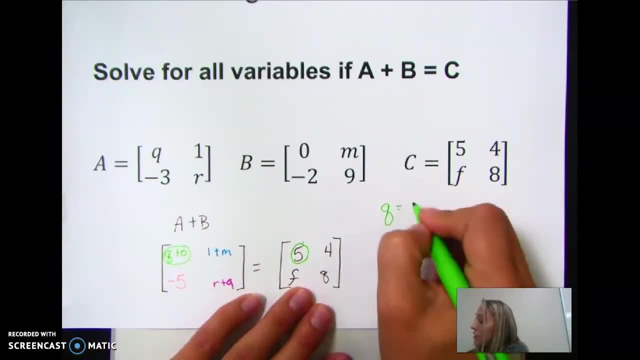 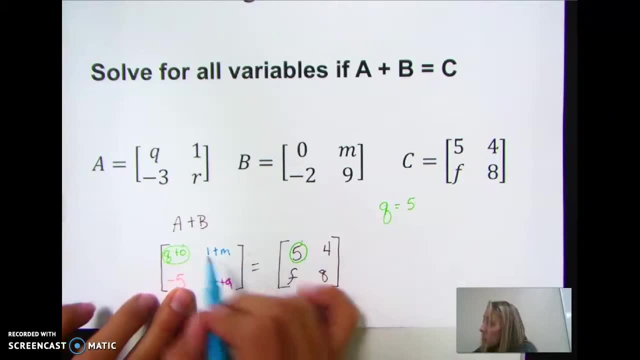 So again, anything plus 0 is itself equals 5.. And that one is done, Then I'm going to do. I'm just going to go to the next one, because it doesn't matter what order you do it in. I could go down here. 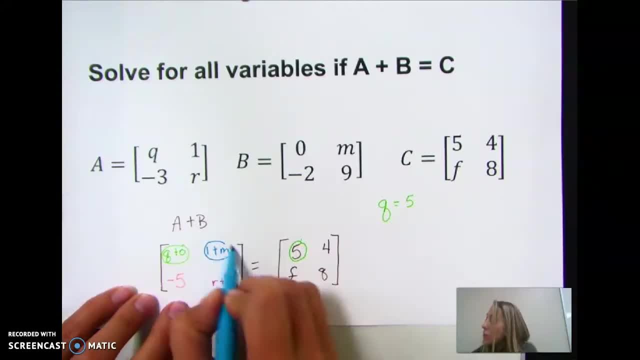 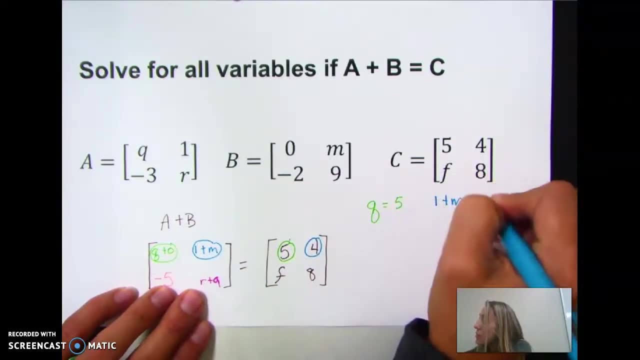 I could go over here, But I just like going right to left. So I'm going to do 1 plus M and set that equal to what's given to me, which is 4.. So 1 plus M is equal to 4.. 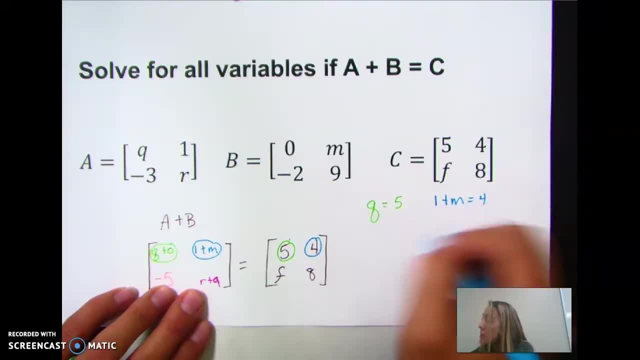 I need my M to be. I need my M to be itself. so the 1 is being added to it And it's a positive 1.. To make that a 0, I'm going to go ahead and subtract 1 from both sides. 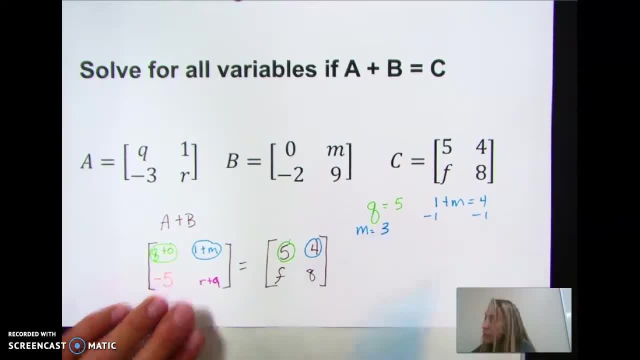 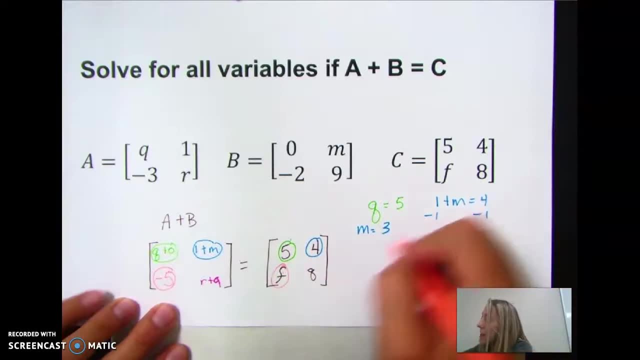 And I'm left with M is equal to 3.. Okay, Now we're going to do that with the negative 5.. Negative 5 is equal to F, So negative 5 is equal to F. That one's easy and that one's done. 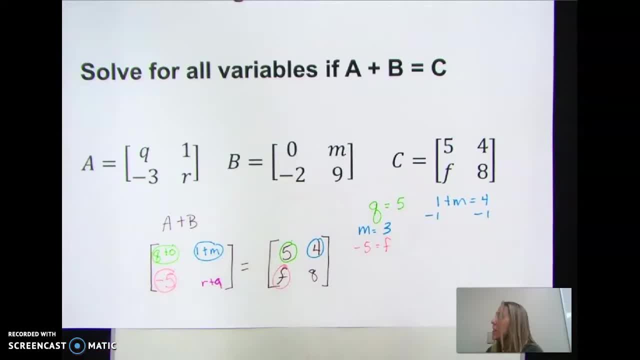 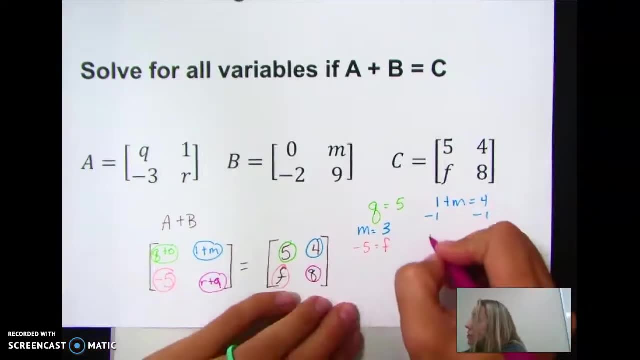 That was almost as easy as the Q, because I didn't have to add anything to it. You could also write F: Negative 5 is equal to negative 5.. And then I have this one, so R plus 9 is equal to 8.. 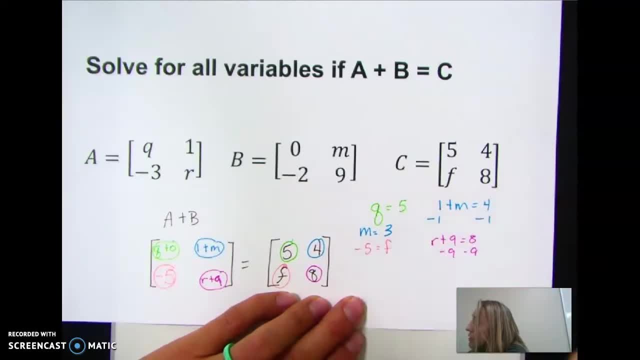 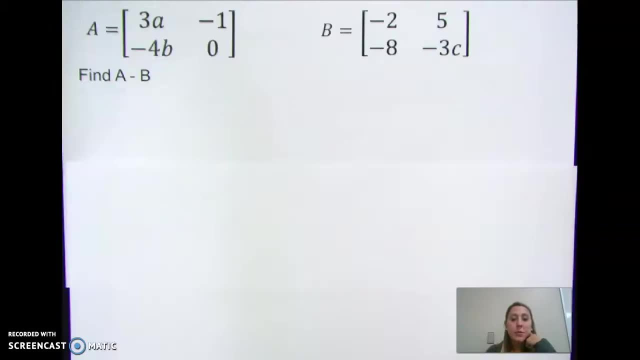 I'm going to subtract 9 from both places, both sides. It gives me a 0, and I am left with R is equal to negative 1.. Okay, so now I'm going to subtract two matrices And I am given A and B and I need to subtract it.